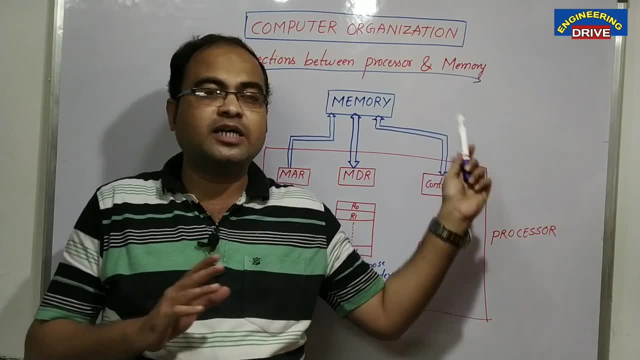 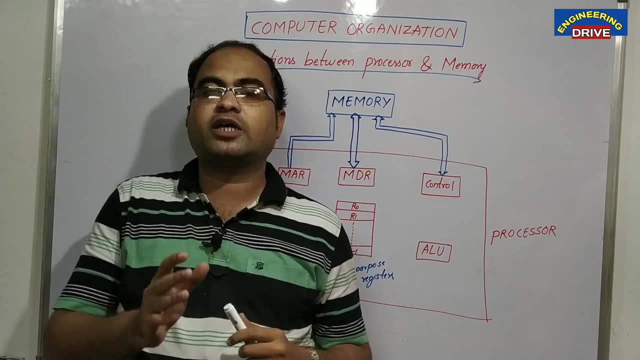 between them. So here, when I am talking about memory, it doesn't mean the hard disk. here It means that whenever I am talking about processor and memory communication, you should always think that we are talking about main memory, that is, RAM. connections between processor and RAM, how our 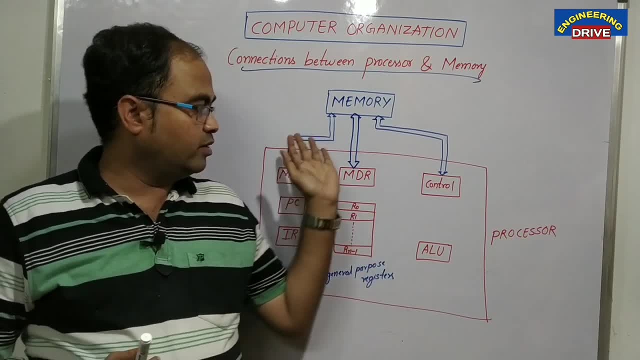 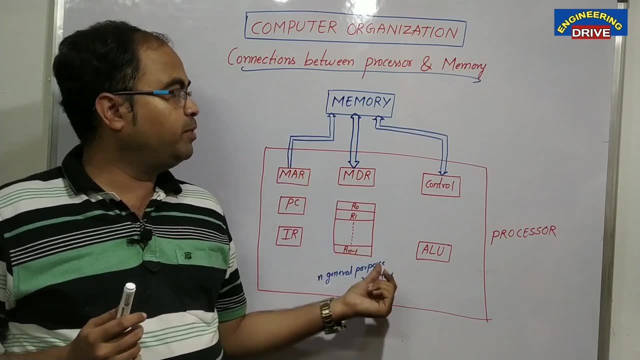 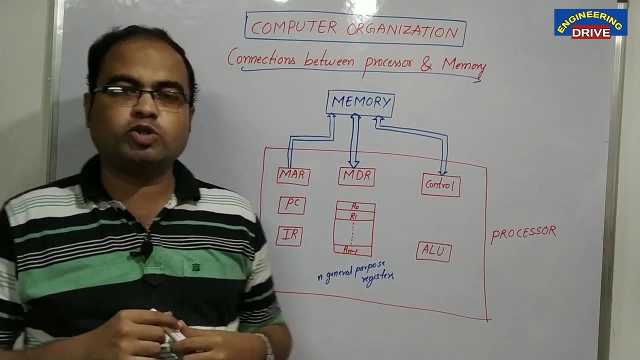 processor and main memory will communicate with each other. So with the help of this very nice diagram, I am going to explain you the communication that will take place between CPU and main memory. So memory here refers to main memory. So you can see here in my previous set of videos you might have watched, simply I 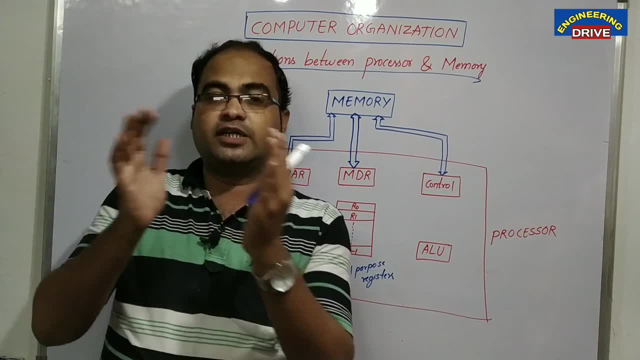 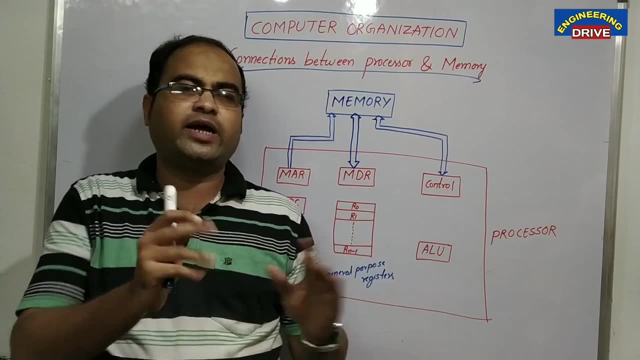 told that initially the data will be available in hard disk. From hard disk it is brought into RAM, From RAM it is brought into cache memory and from cache memory to CPU. Now, here we have not included the cache memory and hard disk. Our main purpose is how the communication will take place from main. 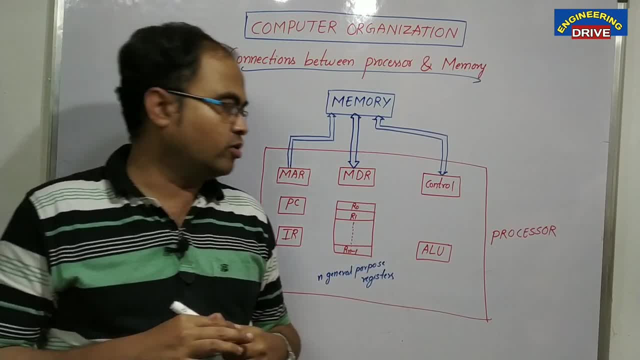 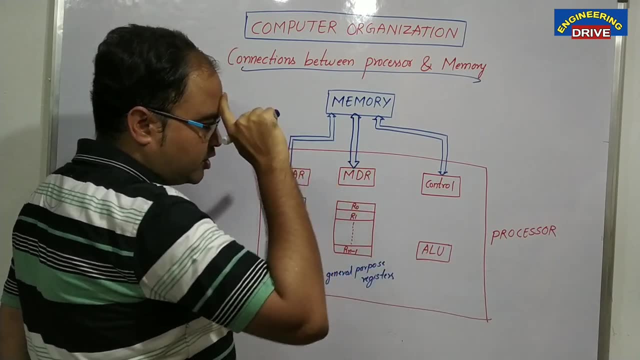 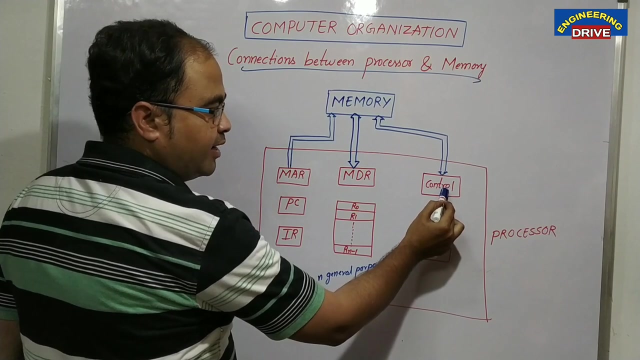 memory to processor that I am going to show here. Oh, okay, So let us say this is our entire processor. Generally in our processor we know that in our CPU there are three important parts. One is arithmetic and logic unit, control unit. second part, and what we call this remaining. 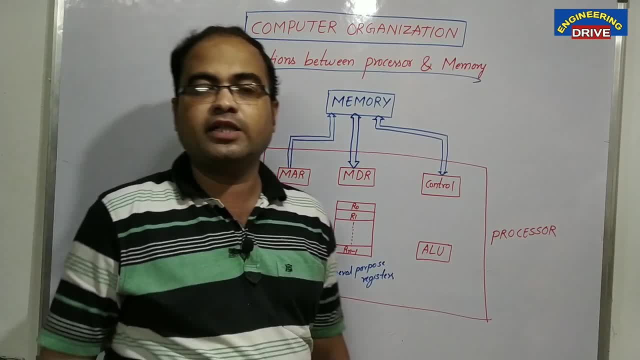 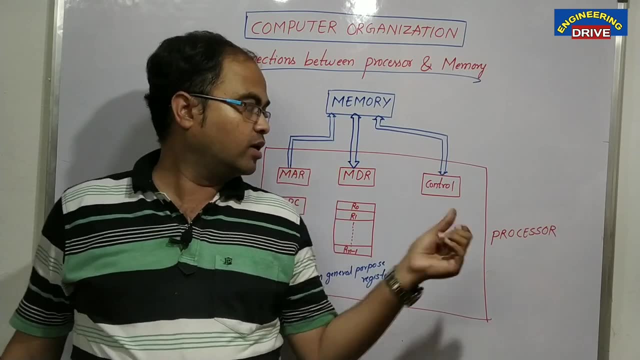 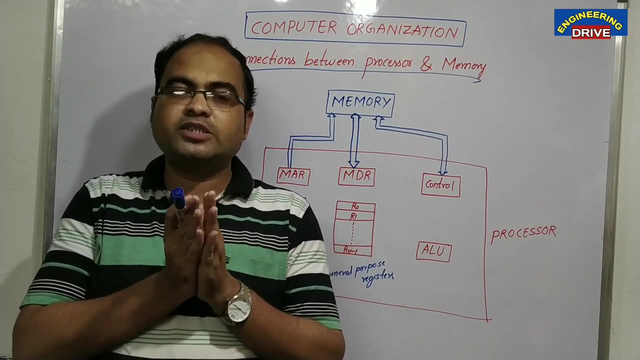 entire part. they are known as registers, What we call them Registers. A CPU contains three parts. One is arithmetic and logic unit. second, one control unit and the third one is we call them as registers. What are registers? Registers are a very small place to store a very small amount of data. 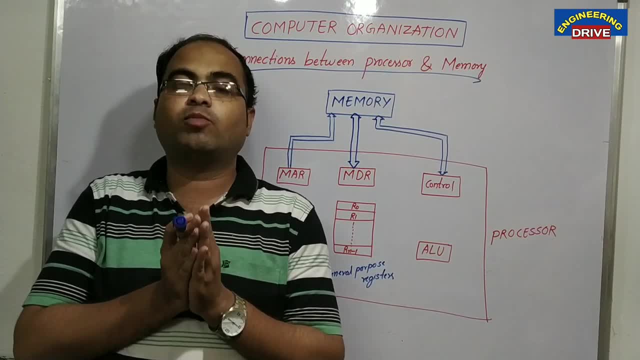 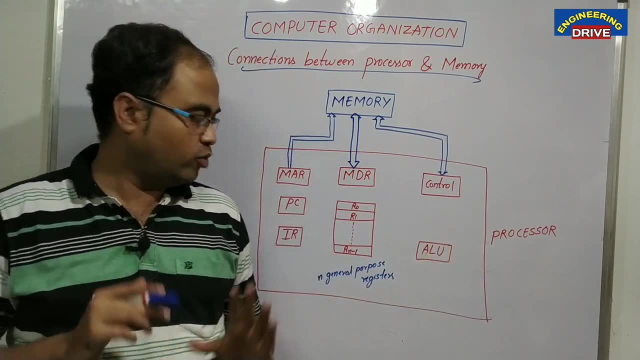 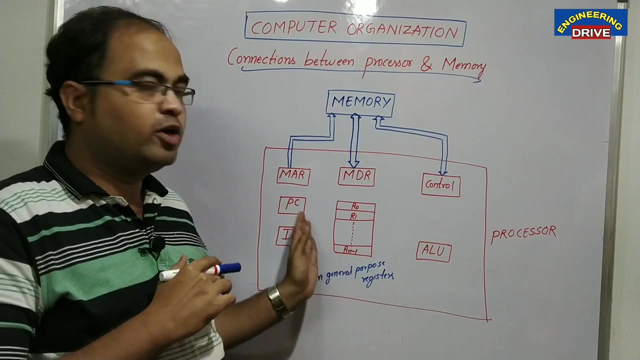 They are not very large in size. They can hold only limited amount of information. So where those registers are available Inside our CPU itself, inside our processor itself. Now, what are the uses of all those registers and how our processor will make use of these? 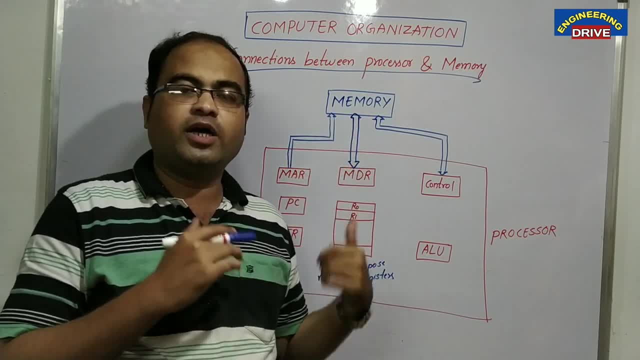 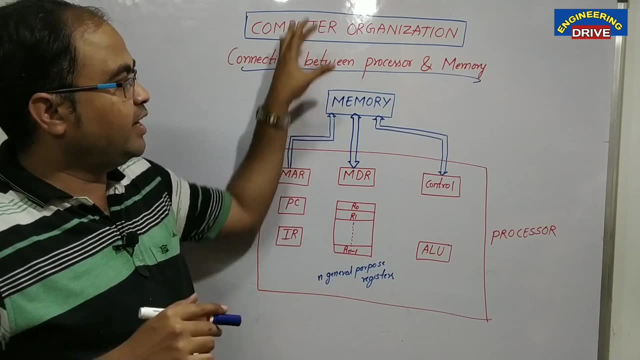 registers in order to access the data from memory or in order to give the data to memory That I am going to discuss here. Let us say initially the data will be in somewhere in hard disk, The data will be brought into main memory. and now what our CPU will do. 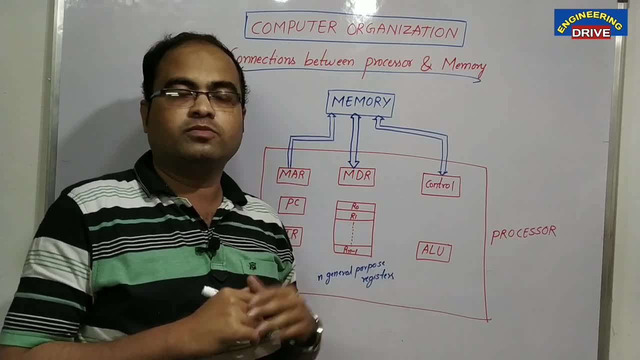 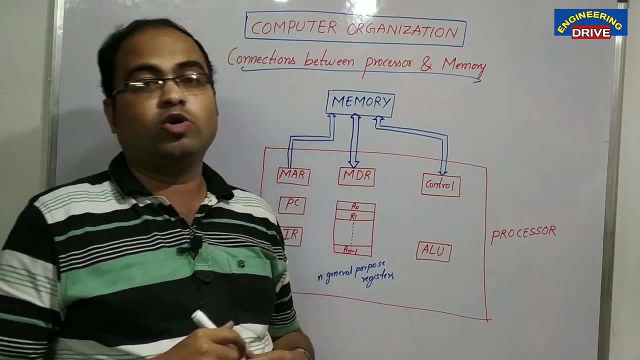 From main memory, the data will be brought to CPU. I told in many times in my previous videos that simply, I told that data will be brought into CPU Where the data will be stored. now I told you our CPU will execute the data in the form of instructions. 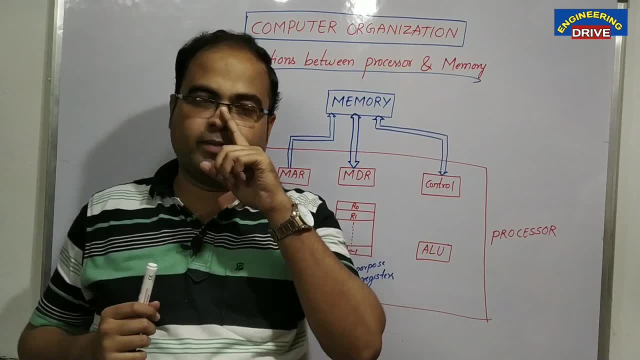 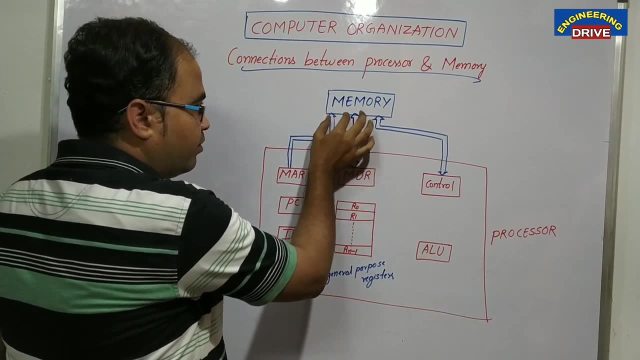 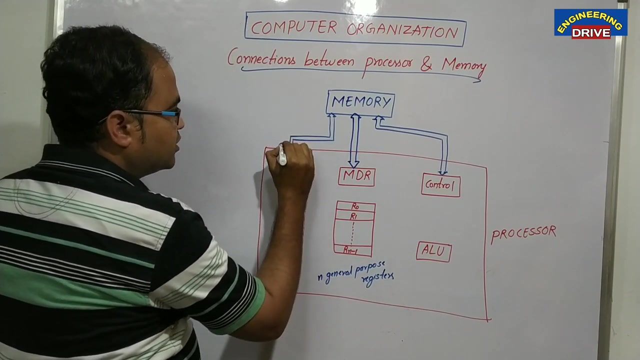 This is very, very important point. It won't execute entire program at a time. CPU will execute instruction wise, Which means when our processor will fetch the first instruction from memory what happened Before that, our processor will specify the address. This is the first step. 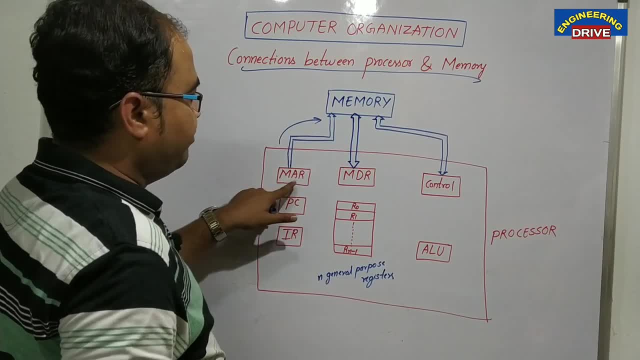 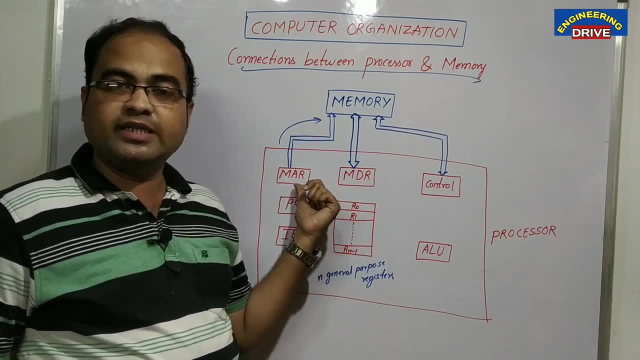 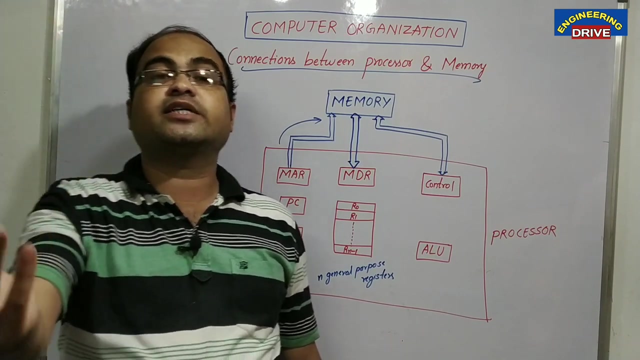 Step number one. What is MAR? This is a register which is available in every processor. MAR stands for Memory Address Register. What is MAR? Memory Address Register Processor will give the first. It will specify where the instruction is available in main memory. 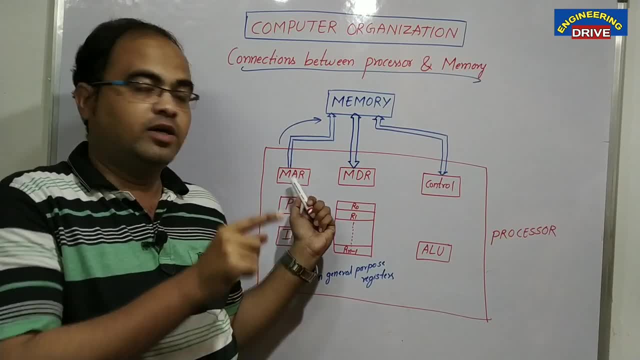 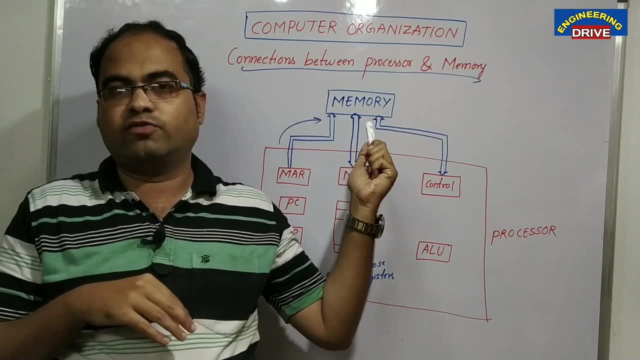 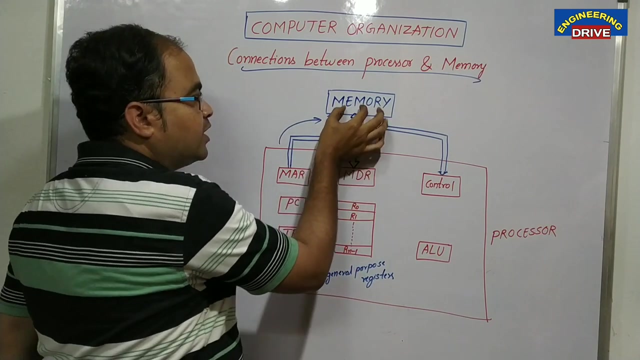 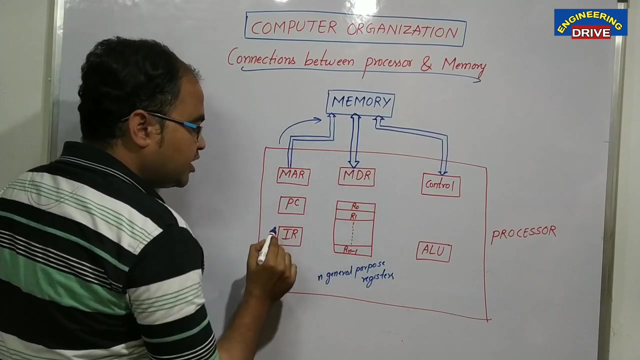 So it will store that address in which register MAR. So MAR contains the address where the instruction is available in main memory Because processor want to take that instruction now for execution. So that address will be stored in memory address register Now. after that the instruction will be brought from main memory and temporarily that instruction 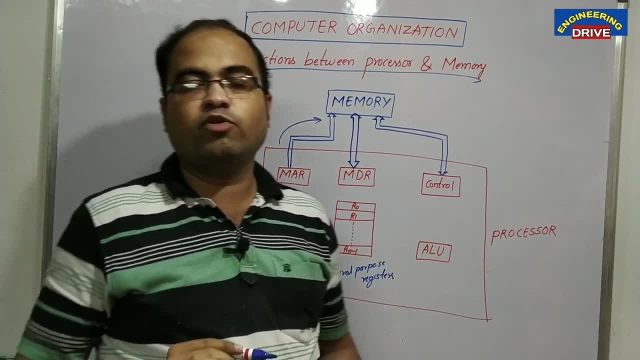 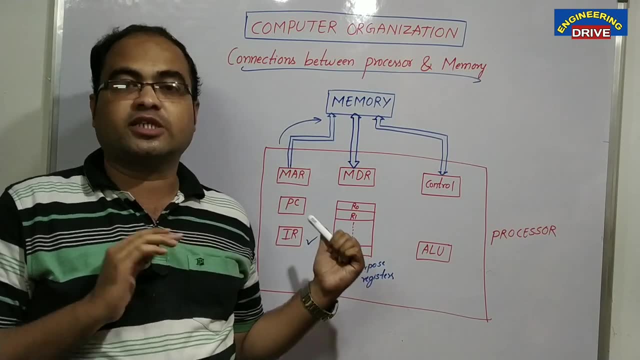 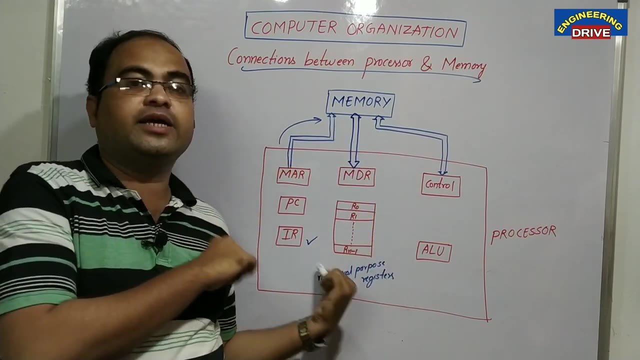 will be stored in 1 register. What is the full form of IR Instruction register? Instruction register stores the currently executed instruction. Whichever the instruction our processor has taken from memory, that instruction will be stored in IR Instruction register. Let us say first: instruction has been fetched. now 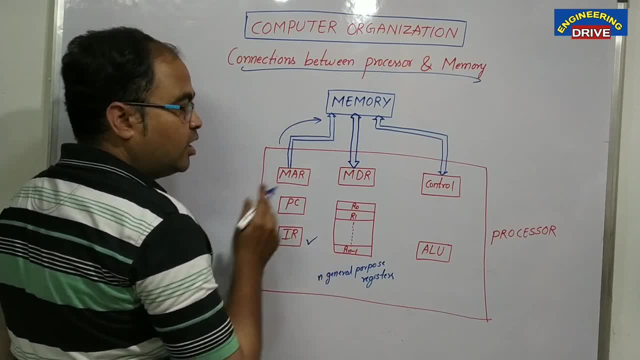 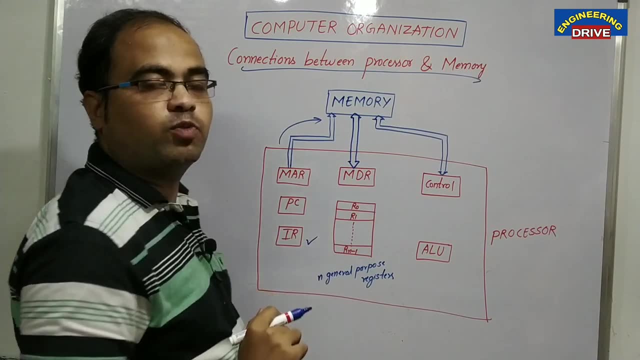 Now, not only that instruction will be stored in instruction register, but also the copy of that instruction will be stored in one more register. Let us call this register as MDR. MDR stands for Memory Data Register. You can see double sided buses here. 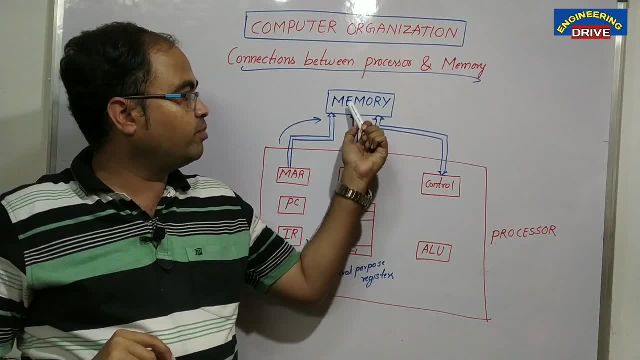 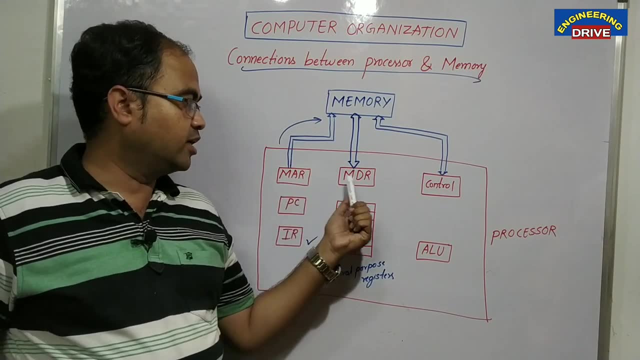 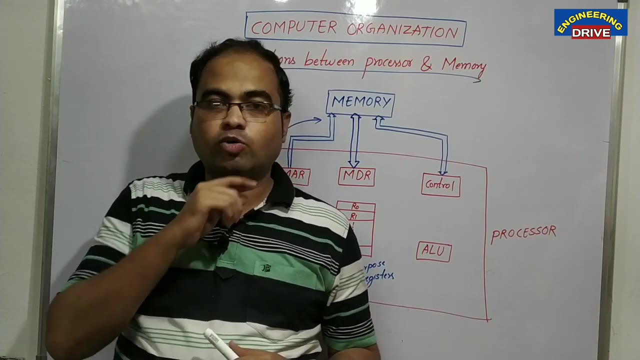 The double sided arrows indicates not only the data will be passed from main memory to MDR, from MDR to main memory also. So MAR stands for Memory Address Register, Memory Data Register, Instruction Register. And what is PC Program Counter? What program counter will do? 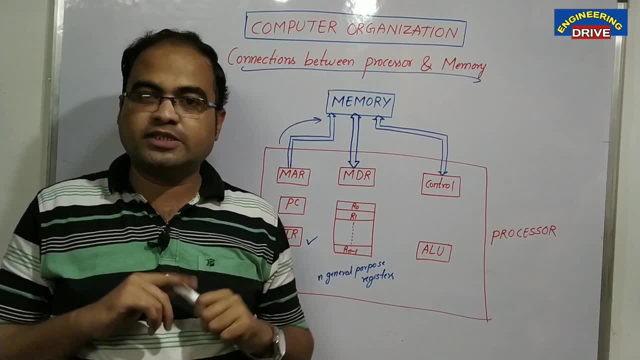 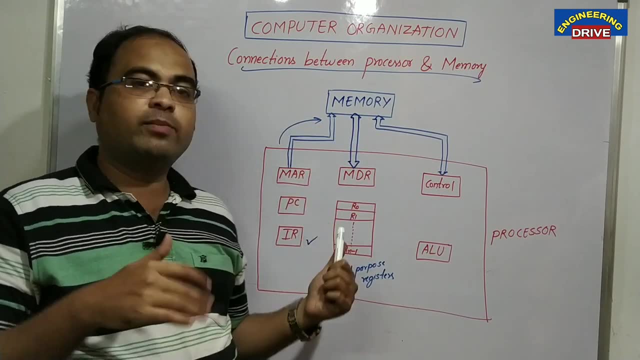 Let us say, first instruction has been fetched now, Then it has been executed successfully, Then the program counter value will become 1.. When second instruction has been executed successfully, program counter will become 2.. Let us say, in our program 10 instructions are there. 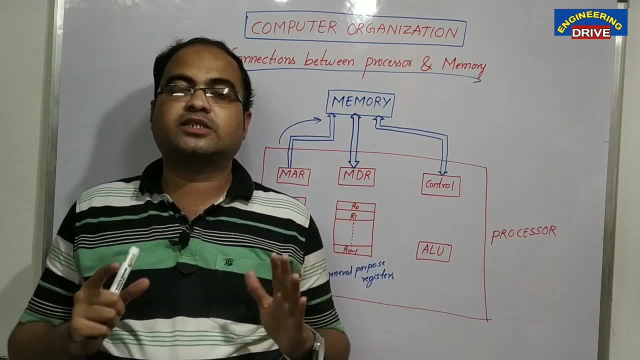 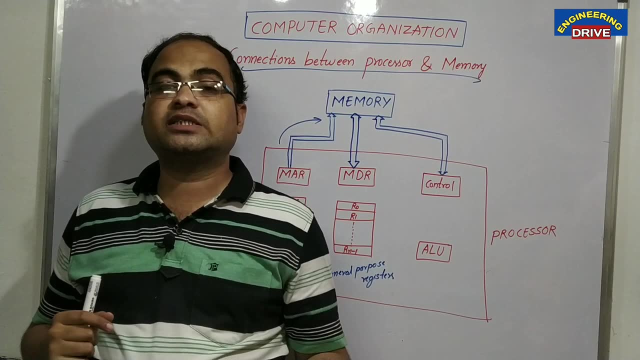 Then the value of program counter will become 10, which means all the 10 instructions have been successfully executed and the final output has came. So program counter will keep track of how many instructions have been successfully executed. That work will be taken care by program counter. 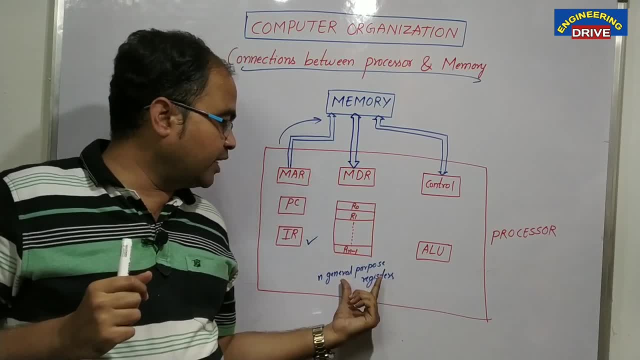 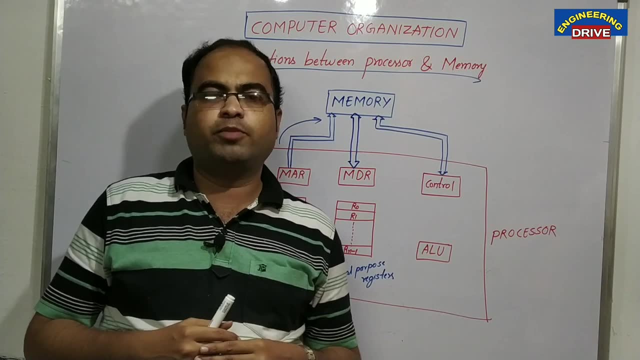 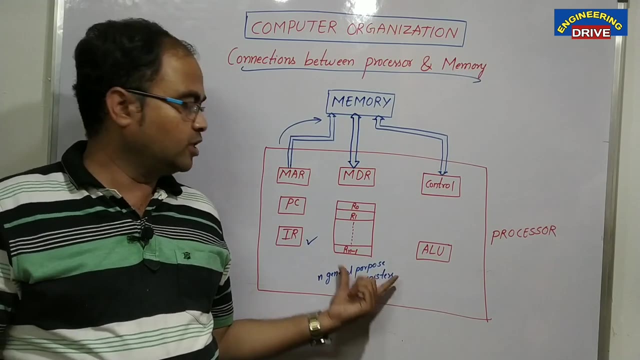 And These inbuilt registers there are from general purpose registers also. We call them as N general purpose registers. There will be, depending on our computer, Okay, Computer's hardware architecture or our CPU architecture, There will be N number of general purpose registers. 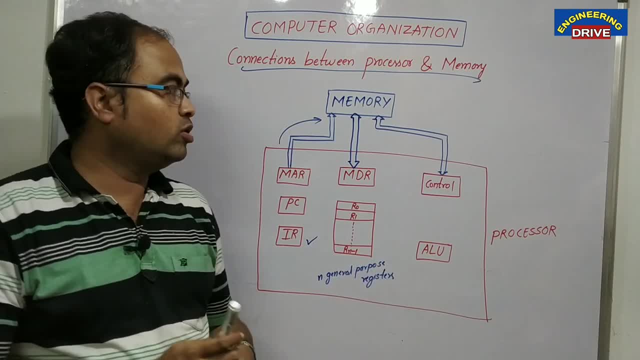 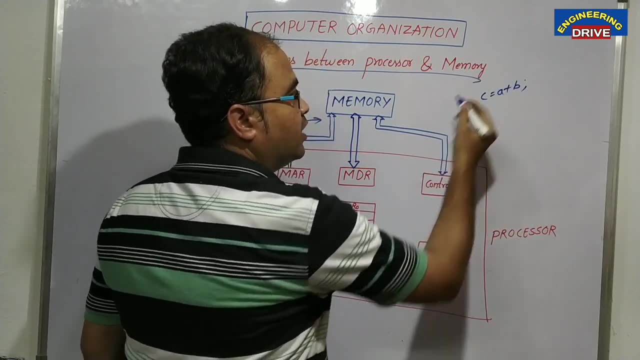 What are the purpose of, what is the main purpose of using these registers? You know, when we write some programs. let us say I have written one instruction in our C language. C is equal to A plus B. Then the value of A will be stored in one register. 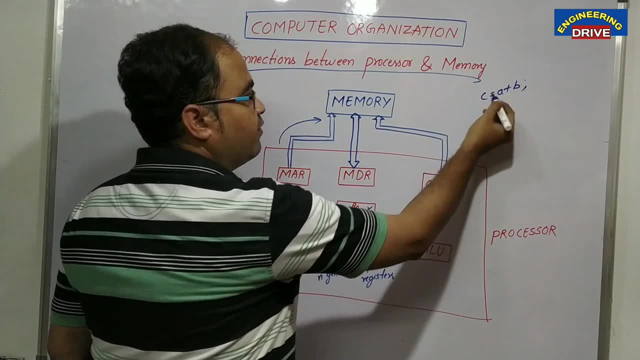 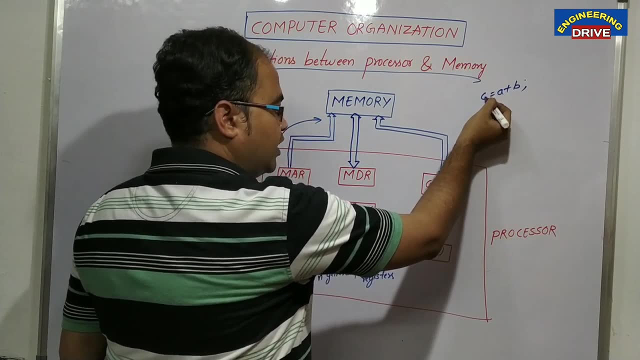 Then the value of A will be stored in one register. Then the value of A will be stored in one register, R-not. the value of B will be stored in one register, R-1.. And finally, the result of C. whatever the result will be assigned to C, it will be: 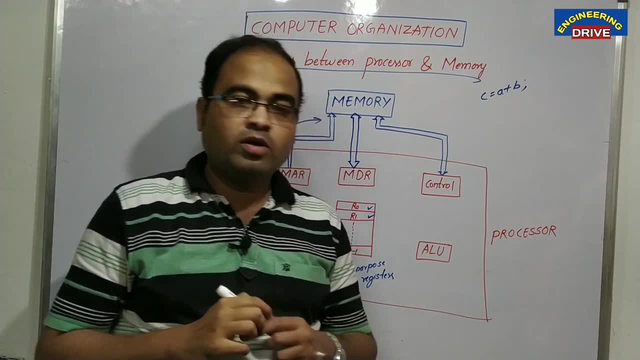 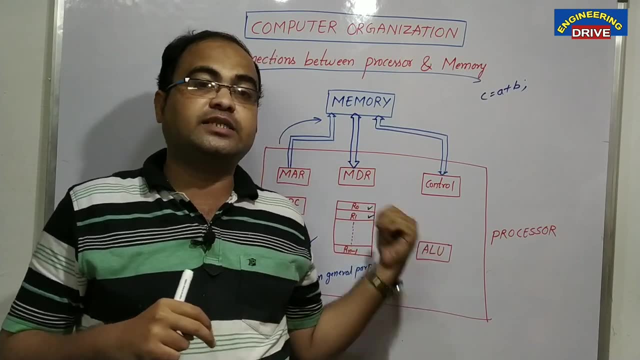 it will be stored in some more register R-2 like that. So for physically they are variables for us But internally our CPU will store the values of those variables in registers at the time of execution. Hopefully it has been cleared to store the those values. general purpose registers are. 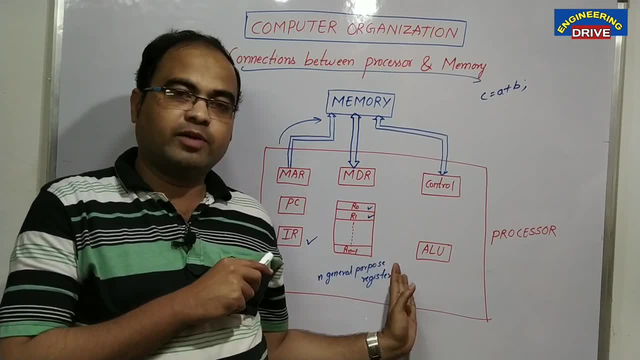 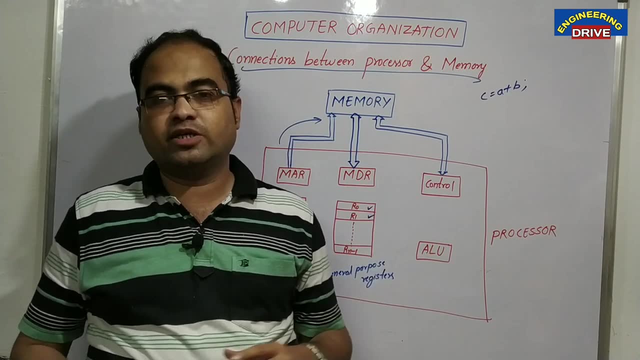 used. Okay, And those general purpose registers. Now the time for calculation. now, Who will do that calculation work? Arithmetic and logic unit will do the calculation work, which means in our case, in this instruction, we need to do which calculation here? Addition, calculation, summation, we need to. 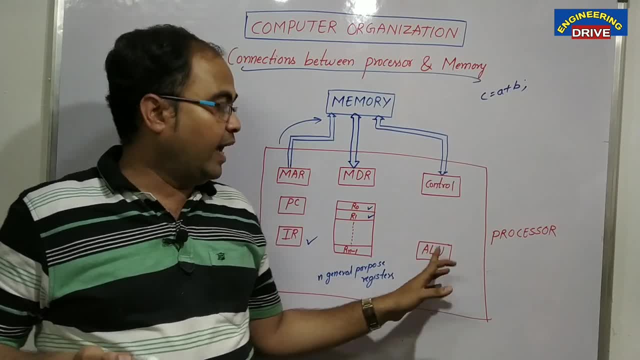 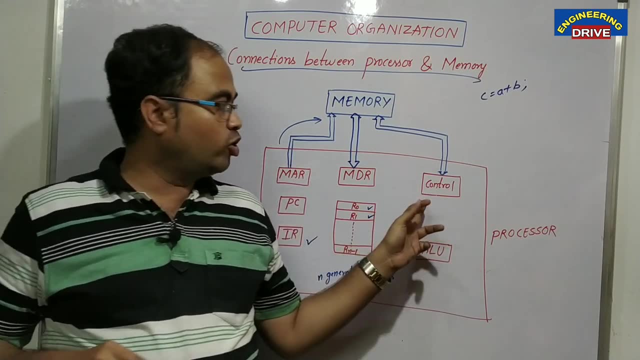 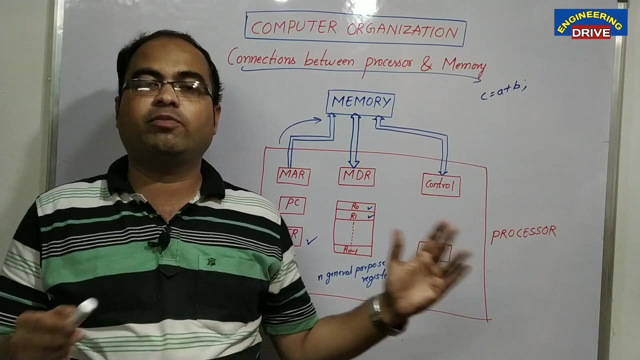 do. That addition will be done by our ALU And this entire work will be handled by our which unit Control unit of our processor Control unit will monitor all these activities. So once again, my dear students, let me once again revise it so that it will be clear to you First from where 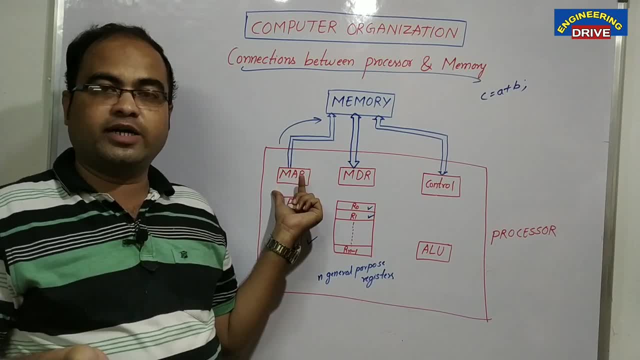 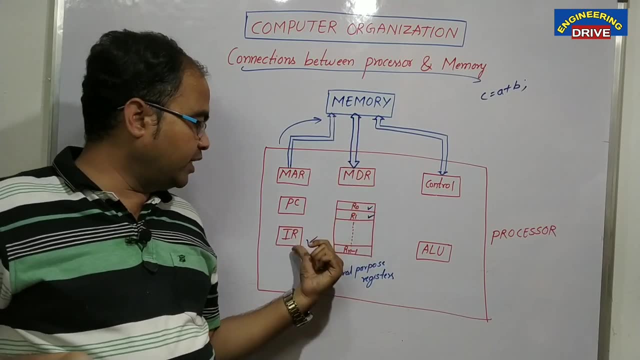 we need to get the data that will be specified in MAR memory address register So that required data will be brought and it is stored in memory data register And the copy of the data will be stored in instruction register at the time of execution And the value of PC will become 1. 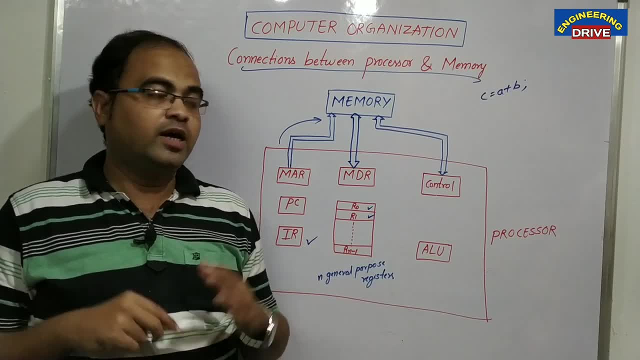 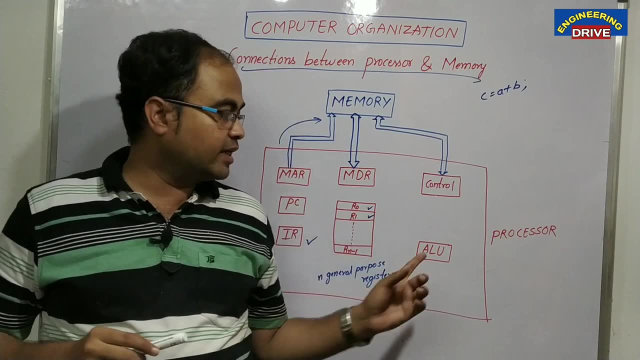 once this particular instruction has been executed And the values of those instructions will be stored in general purpose registers And whenever the time will come for calculation, that calculation work will be taken care by arithmetic and logic unit. And who will monitor all these activities? Our control unit will. 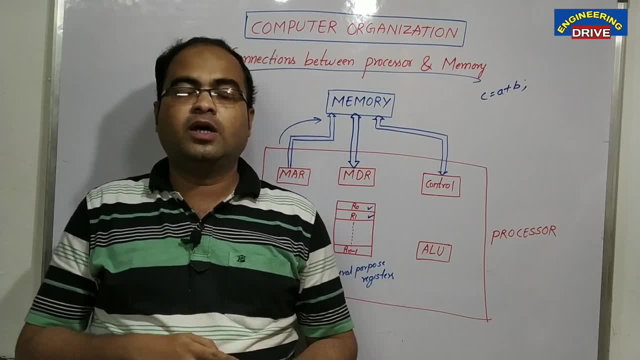 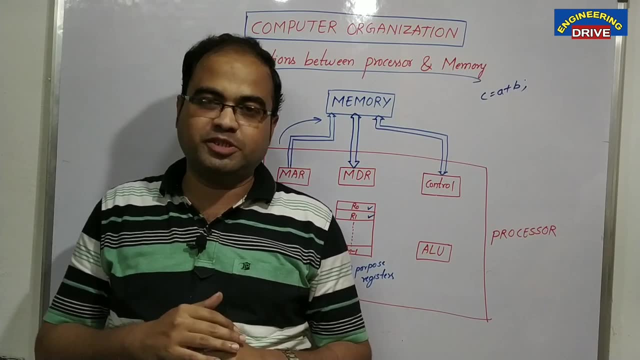 monitor all these activities, See the thing that is going on inside our system. All these things will be behind the scenes We can't see. Once we get the idea of our computer organization subject, then easily we can able to tell what is happening inside our computer. 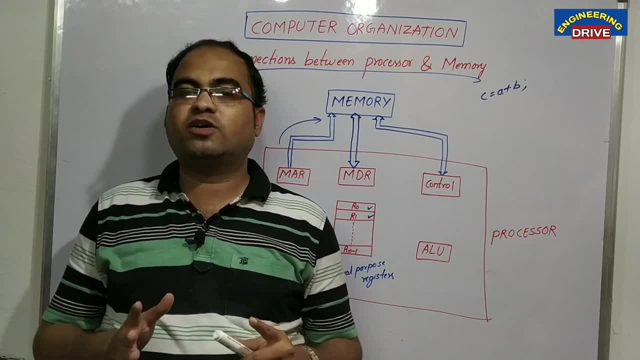 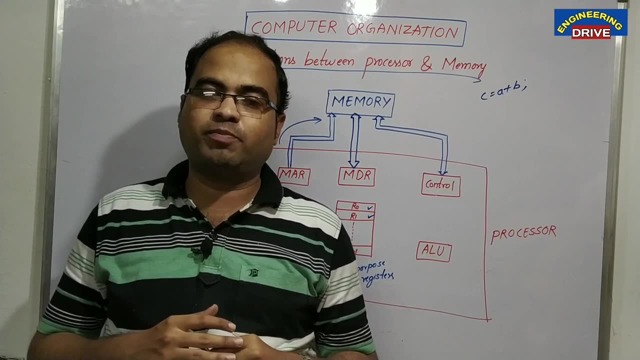 what is happening in our smartphones Easily, we can tell. So the knowledge of computer organization is a must. The knowledge of computer organization is a must For each and every student. OK, hopefully, hopefully, you liked today's topic. We will continue. I will continue more. 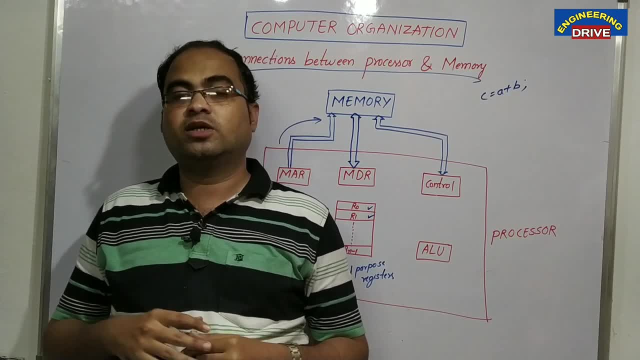 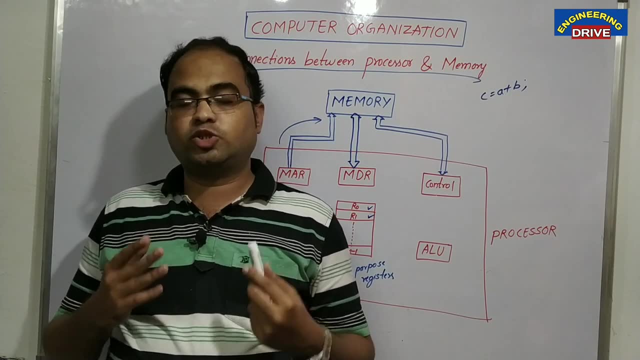 concepts related to addition and subtraction algorithms, multiplication algorithms, division algorithms. Those are also very integral part of our CVO. in my next set of videos, Surely I am going to upload that also. OK, the thing that I am not going to complex concepts. 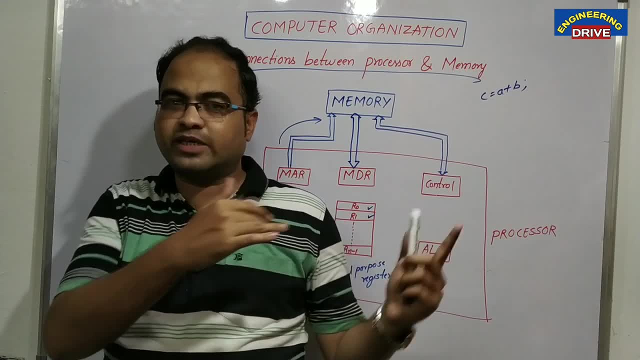 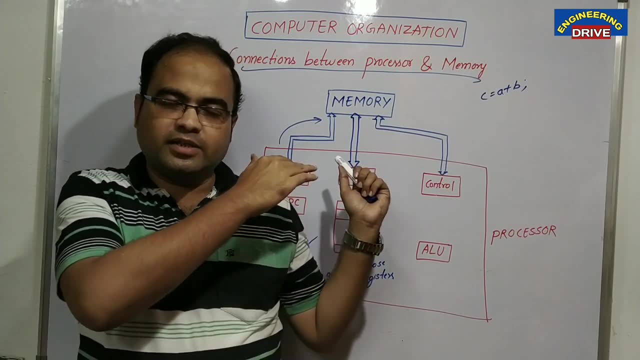 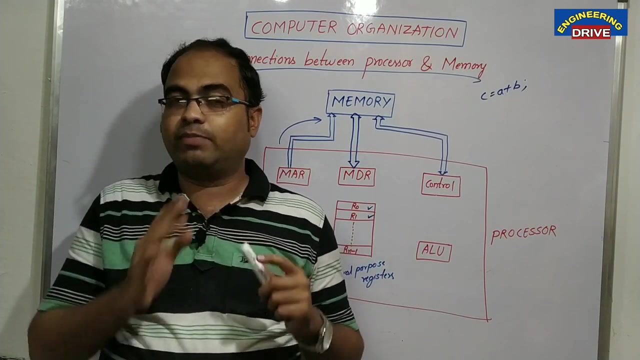 at a time, because there are many students. if you learn from scratch, it will be easy for you. Finally, you can able to solve any complicated problem. that's why let us start. that's why the reason that i have started from basic and slowly i am going to the depth of our ceo and finally, once i will complete the playlist of ceo. 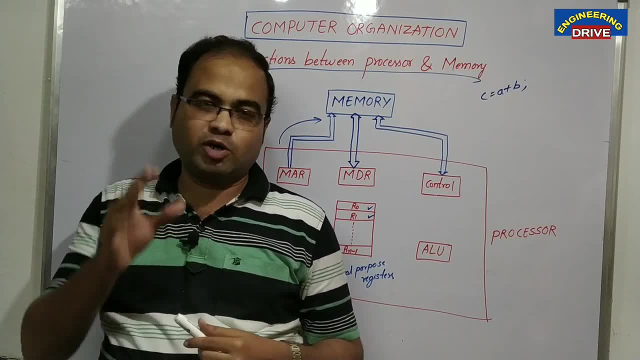 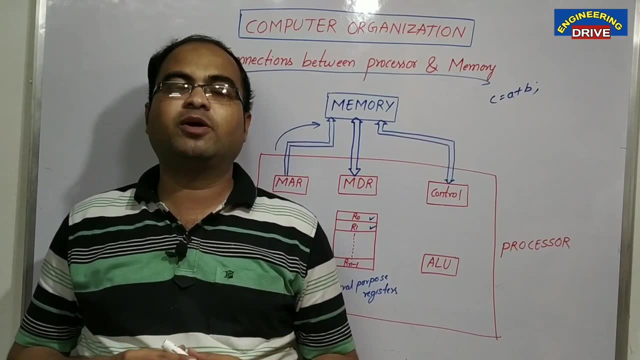 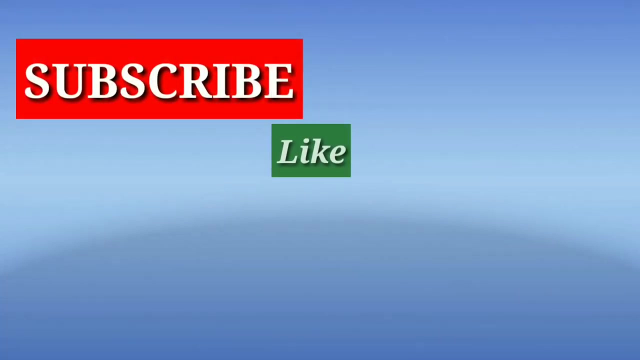 hopefully you will think that how much easy the subject is, because my channel main purpose is to make something very simple for all of you. okay, so with this let me close my today's session of video. see you soon, take care, allah hafiz you.